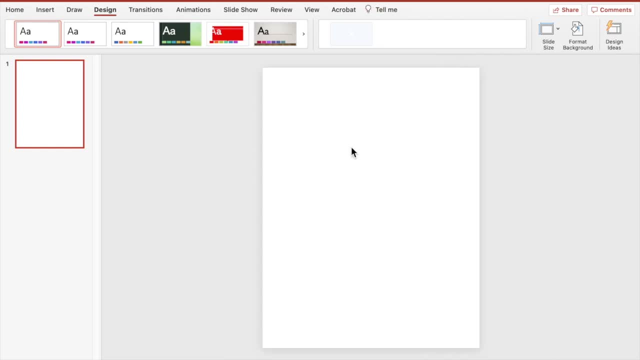 Then we're going to select the page and delete those default text boxes. So what we're going to do, we're going to go up to shape. Now I have shapes as a shortcut in my toolbar, So if you don't have that, just go to insert and then go over to shapes and we're going. 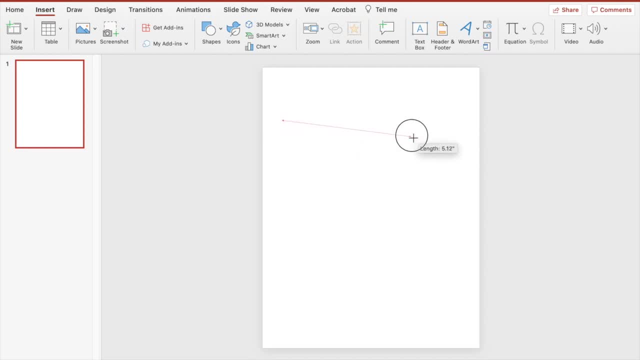 to select the double-sided arrow or double-sided line, And then we're going to make our arrow or our number line, Stretch it out, And then we're going to come up to the line under shape format and make it the color you want and the thickness that you want. 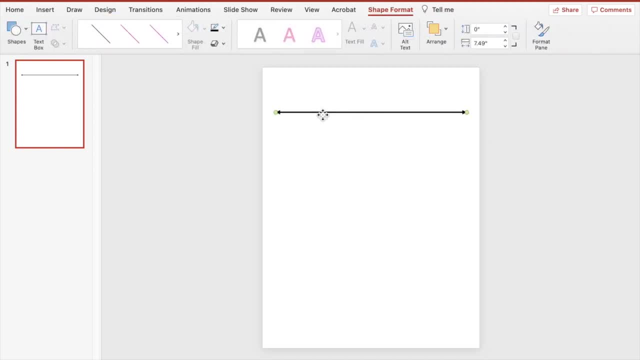 And there we have our first number line. I'm actually going to leave this one like it is, because you can have students using an open number line where they write in the actual numbers that they want to use to solve whatever problem that they're doing. 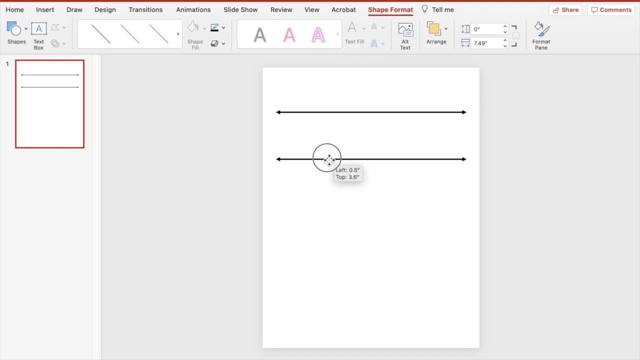 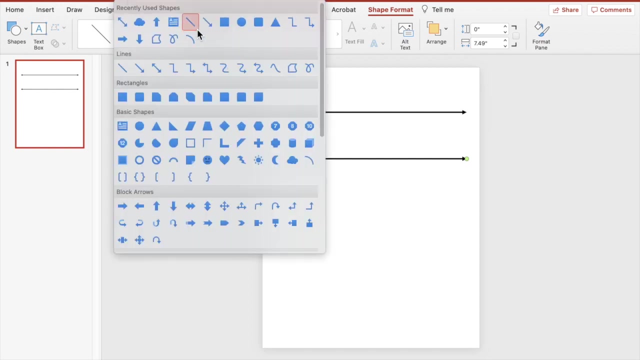 Whether it's adding, subtracting, multiplying or dividing. So let's do another one. Okay, so I duplicated that open number line And for this one we are going to add in tick marks or dashes. So I'm going to come up back to my shape shortcut and select just a regular line without the arrows. 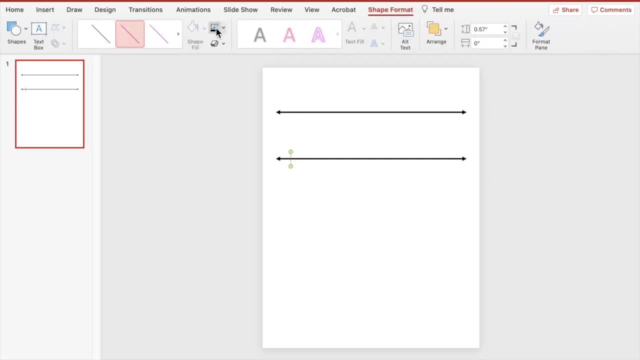 and I'm going to make a tick mark And then I'm going to do the same thing: Change the color, change that shape, the thickness, make it a little thicker and then I'm gonna make it a little shorter. I don't want it to be too long. and if you want to check exactly how, 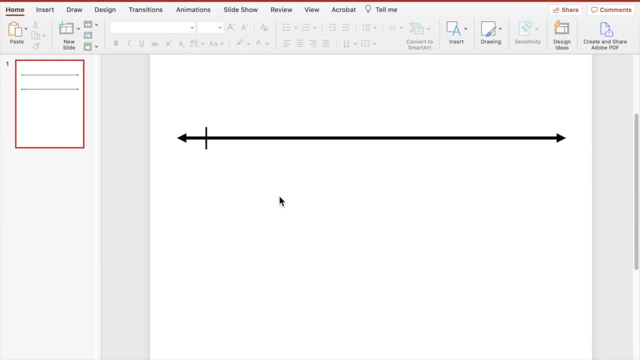 it's laying on that line. just zoom in and I like how that looks. well, let's bring it in to represent our zero, and then we're gonna have it going up to well for our students in kindergarten. let's do one up to five, so that's the. 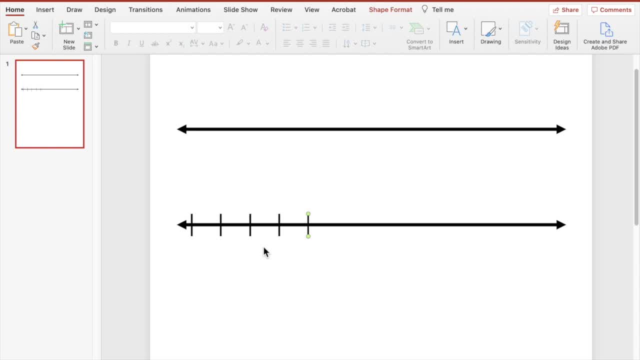 zero. so this would be one, two, three, four, five. now to get it evenly distributed across the number line, I'm just going to move this one down here too. that's going to represent the five. I'm going to select all of the tick marks and they come up here to shape format, go to a range. 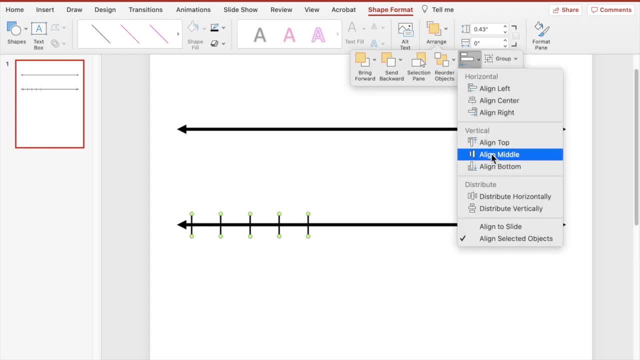 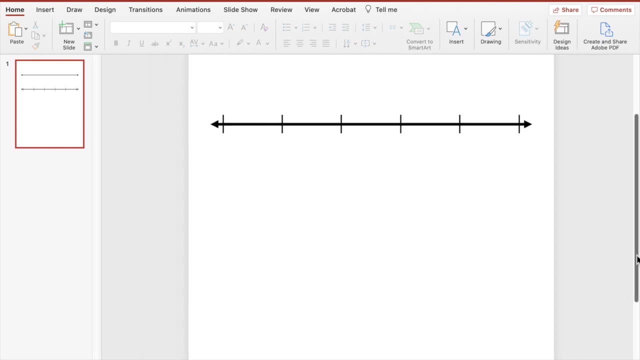 go to a line. I want to make sure they're all leveled in the middle, and then I'm going to go back to a range of line and then distribute horizontally and then they're evenly distributed. so I'm going to do the same thing for zero to ten. so I'm going to duplicate all of that and bring this down and I'm just 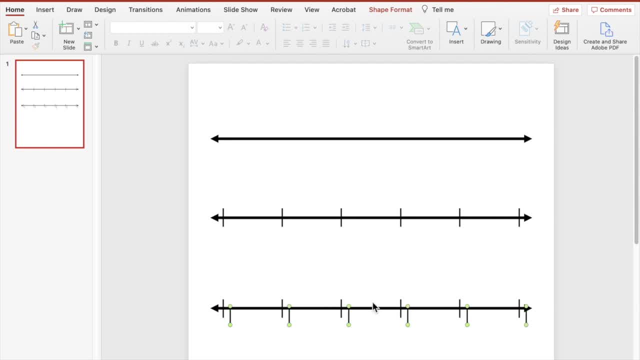 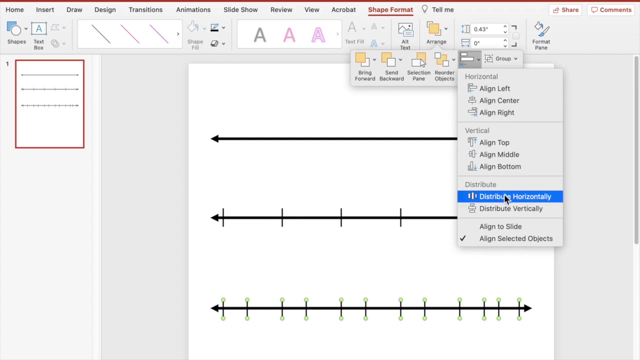 going to select those three and then I'm going to move this one down here and I'm going to do the same thing with the arrange. select all of them. go to shape format. arrange a line. make sure they're all in the middle. arrange a line and. 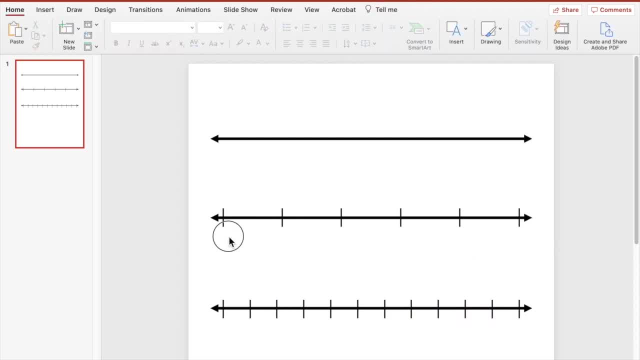 then distribute horizontally. so now we can add in our numbers. so you can leave it like that. or add a line and then distribute horizontally. so now we can add in our numbers. so you can leave it like that or add in numbers. so I'm going to add a text box. put that here, use the font that. 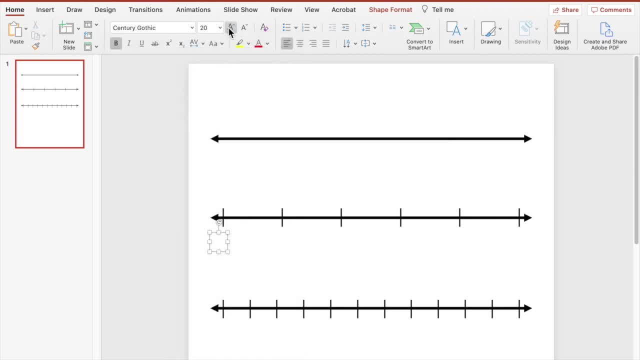 you like and the size that you like. so this is going to be zero and place that there. let's bring it in just a little, and then I'm going to duplicate that and bring it here, and then I'm going to duplicate, duplicate all the way over, and then you can make. 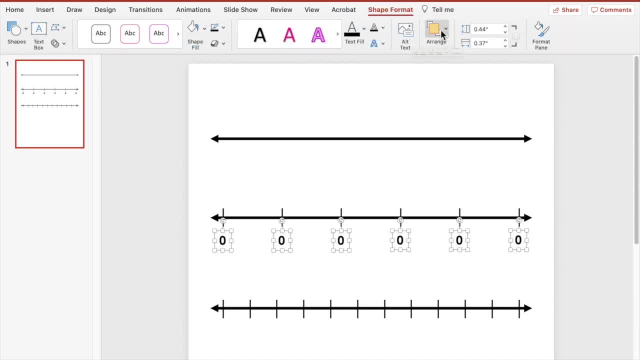 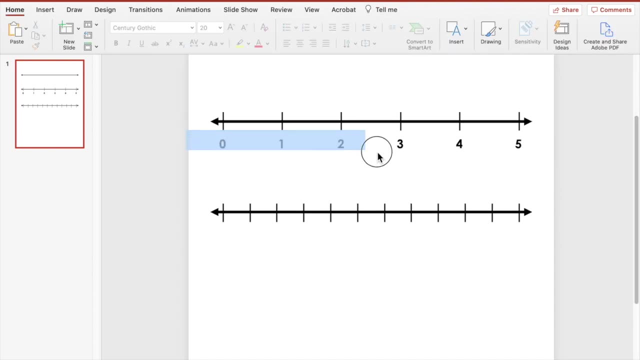 sure it's all, even by going back through the arrange and alignment, and then you just want to change your numbers. so then we're going to do the same thing for the numbers below, just going to take the zero and duplicate that, and then duplicate it like I did with the earlier ones, and then going across. 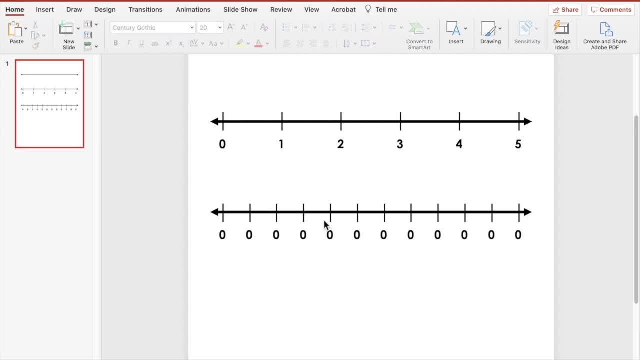 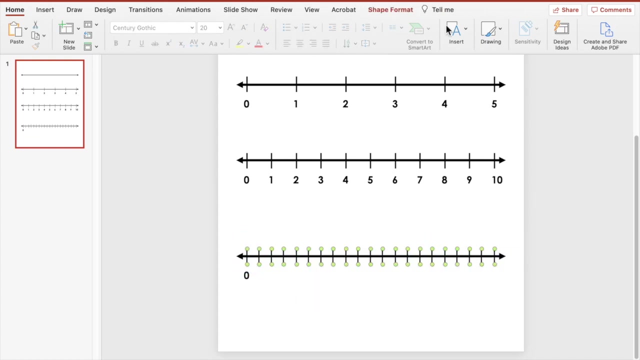 and then going through and changing those numbers, and there you go. so we have our three number lines. let's do one more. let's do one up to 20. we're leaving it free. I can just win that, and that's the way that we have to do it all the way around. just to awesome. so I'm just going to wrap this. 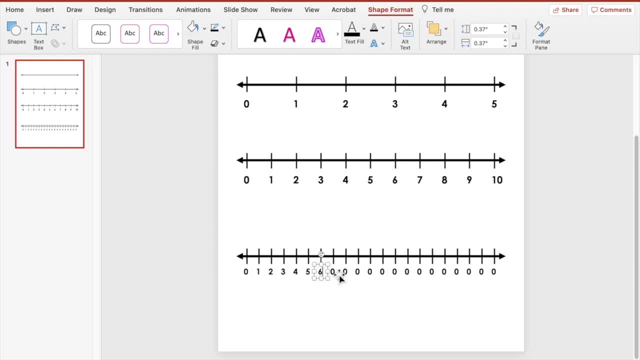 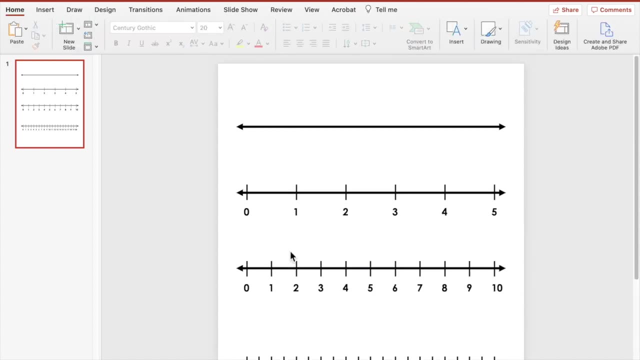 team hair around and then color it off and we'll just drag it over to the inner area to add maximum volume into the side hair. so there you go, there you go. so you got an edge. but this is important. Dennis doesn't want you to see it as it. 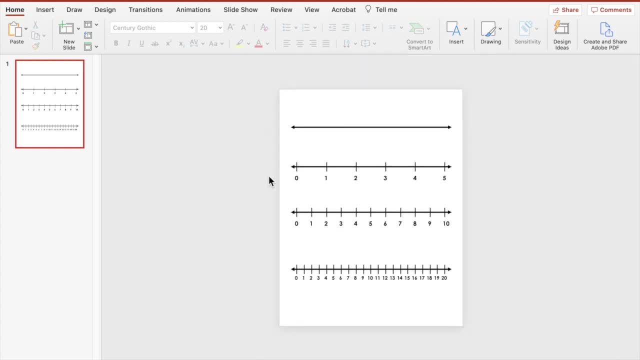 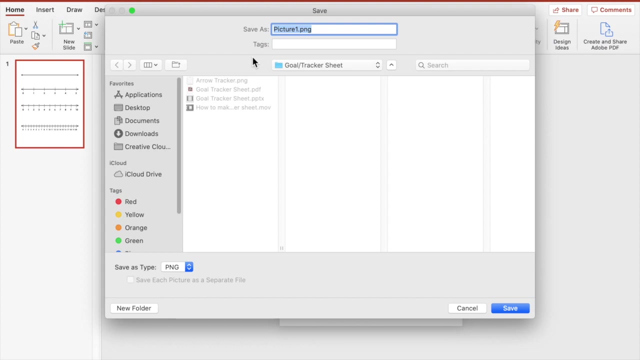 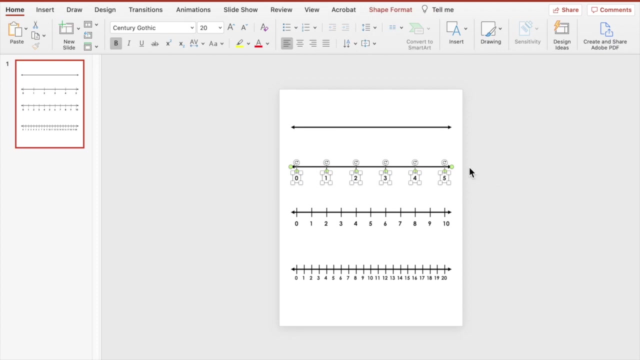 set. so with this resource- I'm not necessarily making a page for students- I wanted to show you how to make your own number line, so I would definitely save these as a picture. so we're gonna select each number line and save them as a picture and save and then make sure we're gonna group these first and then. 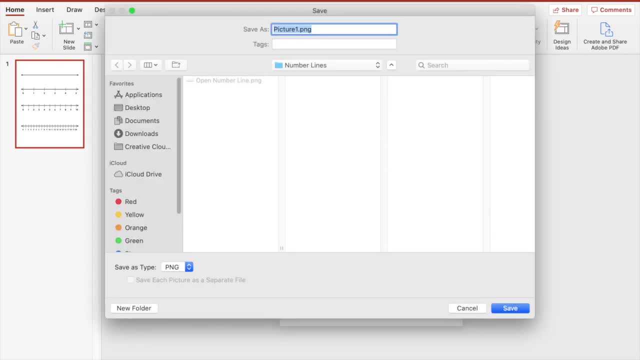 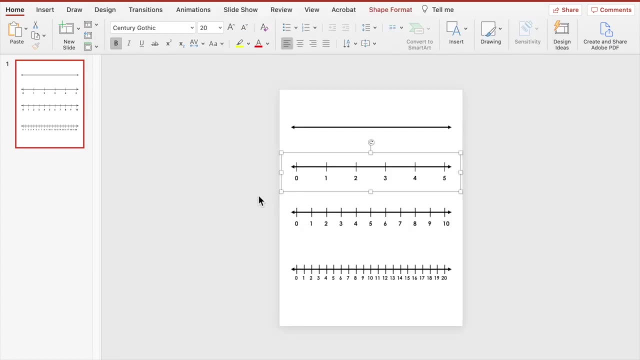 save as a picture. so zero to five number line. so to group them I'm selecting all of them and then hitting right click, right clicking it, then hitting group and then group again, or on your keyboard you can hit command option G to group. so save as picture. 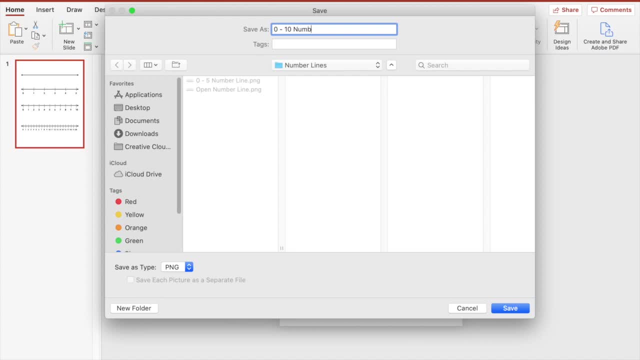 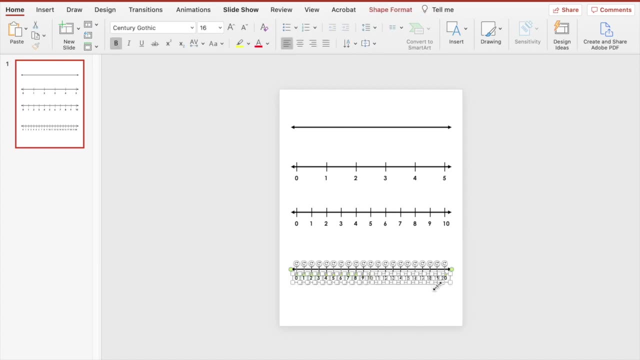 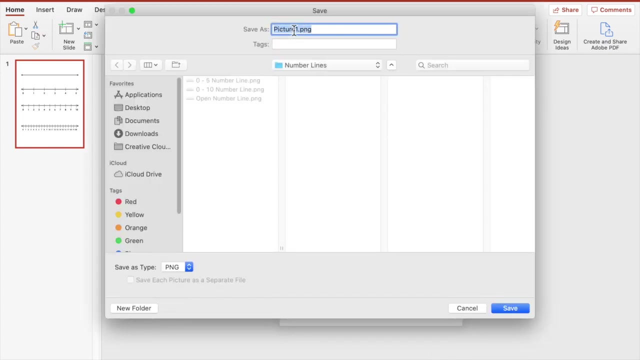 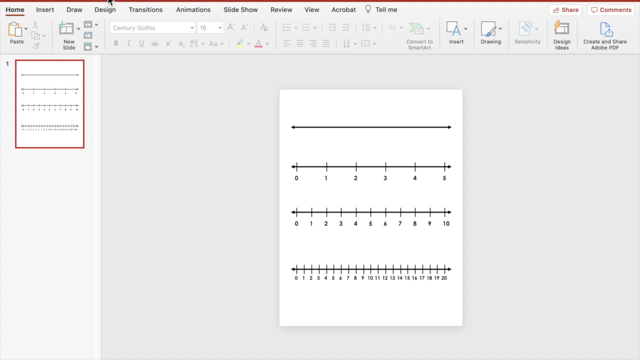 this is zero to ten number line, then this one here: group right-click. save as picture: zero to twenty number line. so just so you know what it is. later on, these number lines can be used to count on, count back using a number line, all right, so let's do a second one here, so I'm going to go ahead and save this one. 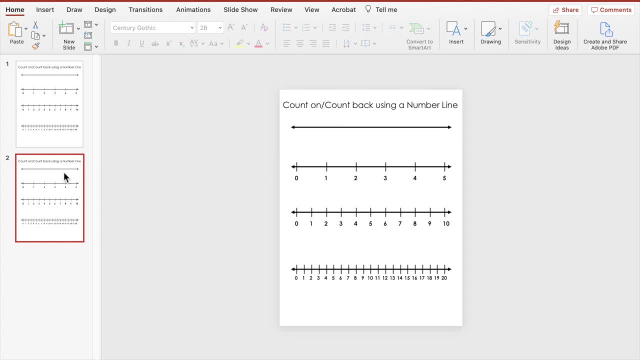 here and I'm going to go ahead and create a second page. so now we're going to look at how we can use the number lines for rounding. so let's keep. we're going to get rid of these two, and this is the bottom one and we're gonna use. 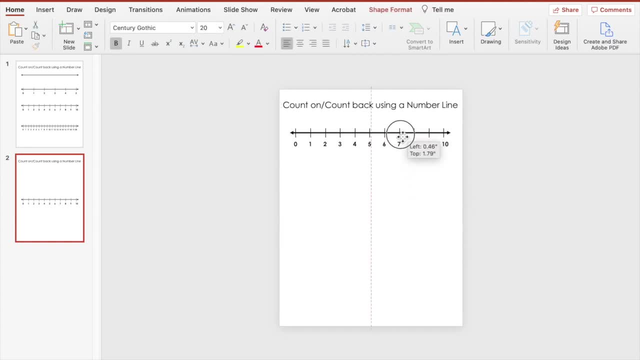 one that goes within ten. so we can use that to round, so that they know we're starting rounding, going between zero and ten, running to the nearest ten. so let's duplicate that and then we're gonna switch out these numbers. so let's make this a 10. I'm going. 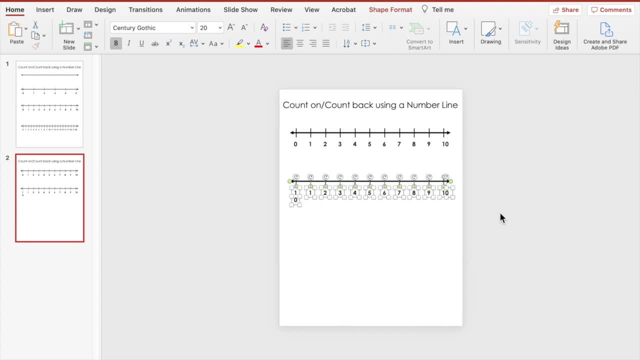 to ungroup it group ungroup, and then I'm gonna select the text boxes in between my tens, so that's gonna be 10, and then I'm gonna change this to a 20 so students can figure out, like, where to place their number and how to round to the nearest. 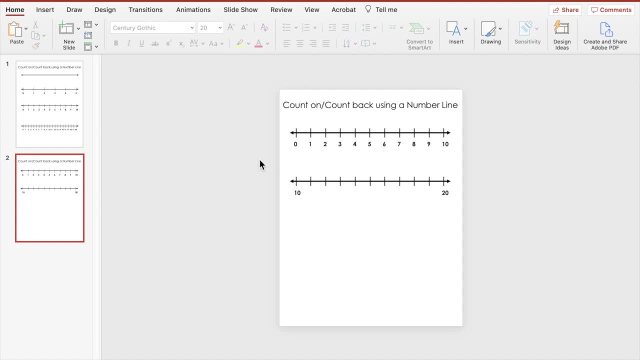 10, if in between, if it's between 10 and 20, we can do the same thing for a larger number. so like what, if we did 100 and this was 200, we can do that, and you can do one where you give the students the midpoint, because some students struggle. 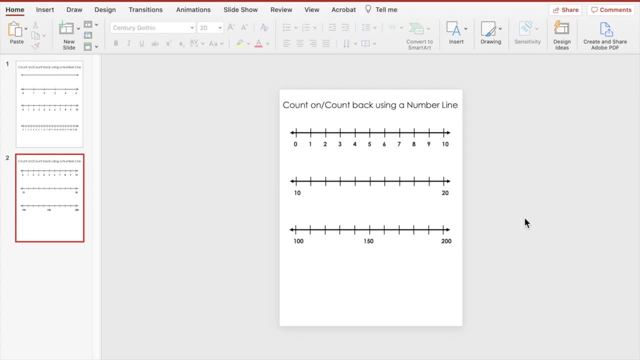 with figuring out the midpoint. have you given them midpoint around, or if their task? maybe let's see if it's a higher number. let's say 470, this would be 480. so then, instead of giving them the midpoint, you can put a question mark and see if they can figure out what that midpoint is. what is the middle point? 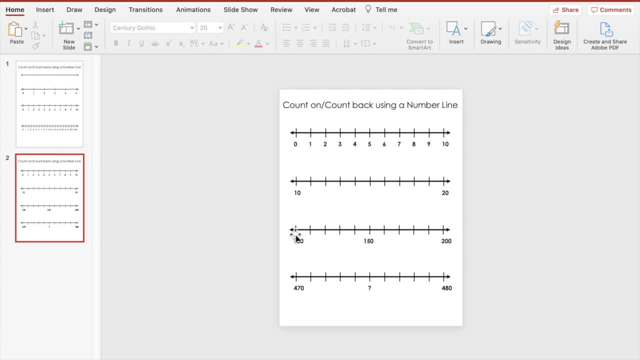 between 470 and 480. so the there are four different types of number lines to use to help students with rounding using a number line. and let's save these, group them and then put them in the middle, and then put them in the middle and then save them as an picture and save so we have all those as pictures, okay, so let's. 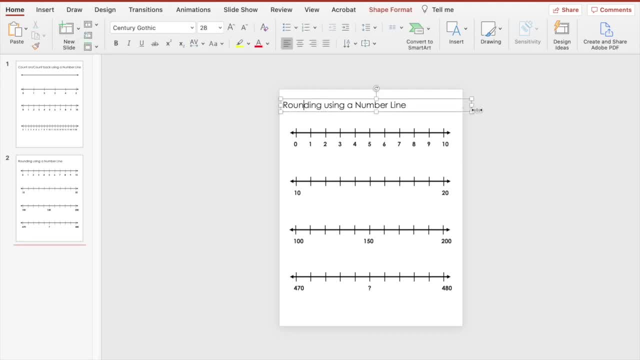 do another one, let's move this down and let's duplicate this page. then this last one is going to be fractions on a number line. so what we're going to do, we're going to get rid of these and we're actually going to go back to that first page we made and copy that open number line and leave that. 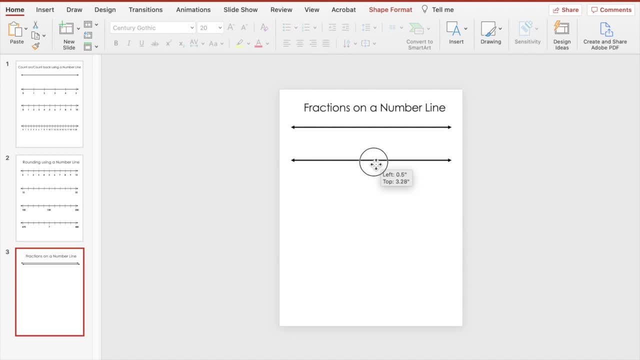 there and then we're going to duplicate that and we're going to add in text box to represent the zero and the one, make it bold, centered. we're going to have a space for the one like one whole, alright, and then we need to bring in our tick mark so we can recreate that tick mark or we can. 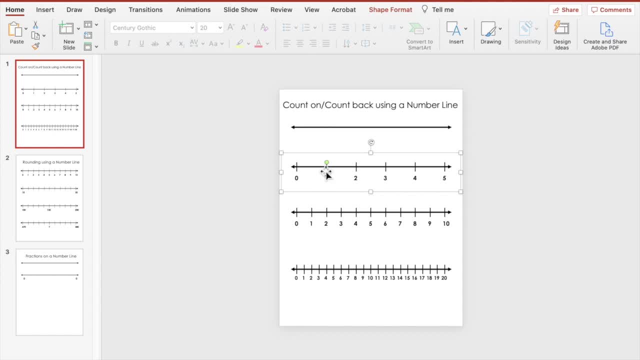 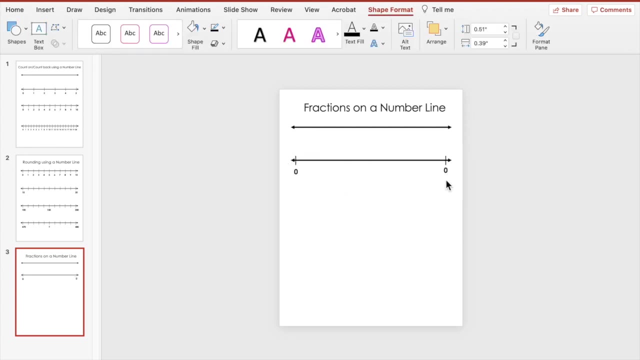 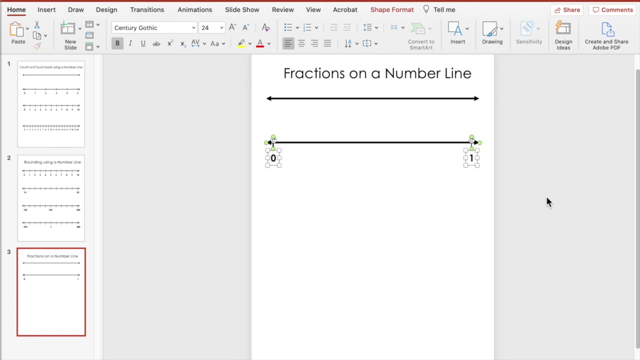 just pull from one of the ones that we already made, so copy and then paste. that's pasted two times, and then we're going to put those as our end points and we're going to change this to a one. so now, what if we wanted this number line? but we wanted 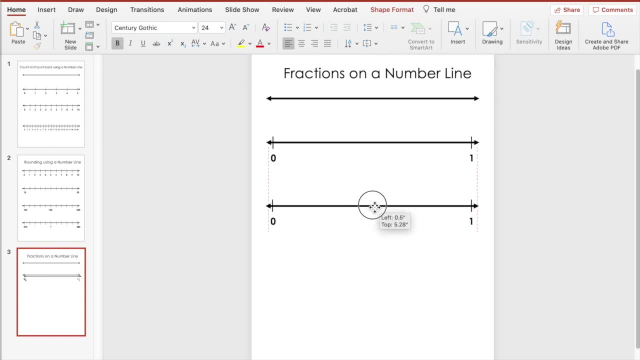 to show the half mark. so I duplicated that. and then I'm going to grab one of these tick marks and duplicate and then bring it in the middle. grab the wrong thing, bring that in the middle and then we can distribute horizontally. okay, perfect, you can leave that blank. so 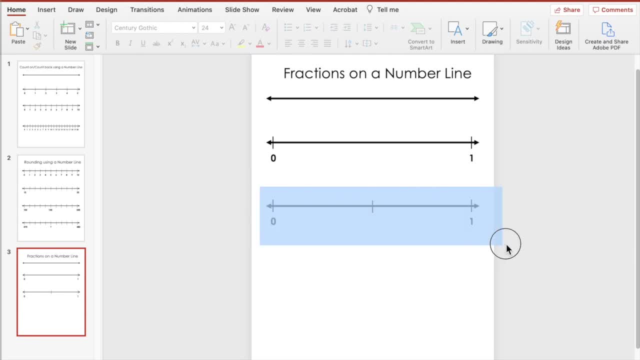 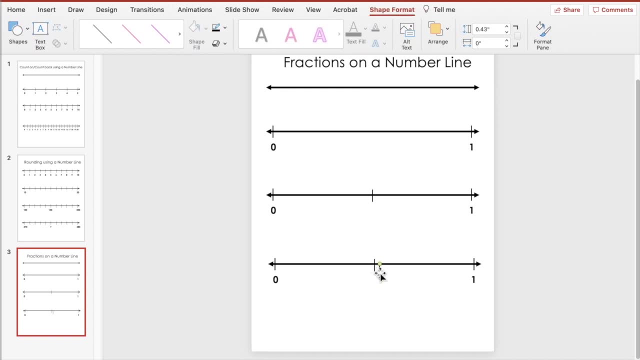 students need to figure out that. that's the halfway mark. let's duplicate this. take the tick mark and duplicate it twice. put one here, one there. don't worry about getting it perfectly in the middle, because we have that alignment button- align- distribute horizontally. and then we have our fourths, and then we're going to do this one. 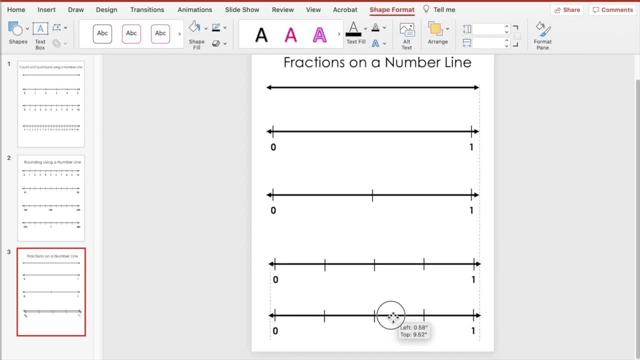 more time I could do eighths, but let's look at what thirds would look like. so we are going to take these lines and actually let's take one out and okay, so redistribute, and there we have our third. so I'm going to move these up. let's go ahead and group these. 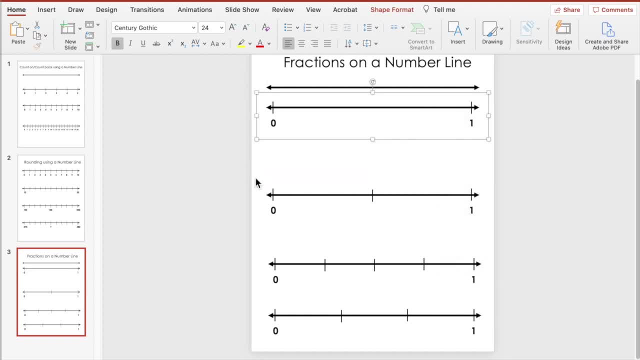 move it up. so with your fractions on your number line. one task students can work on is just figuring out, okay, based on how the number line is going to be distributed, the number line is partitioned: what? what's the denominator? what fraction size pieces are represented here? so there are three equal pieces of the whole. so that means there are thirds you. 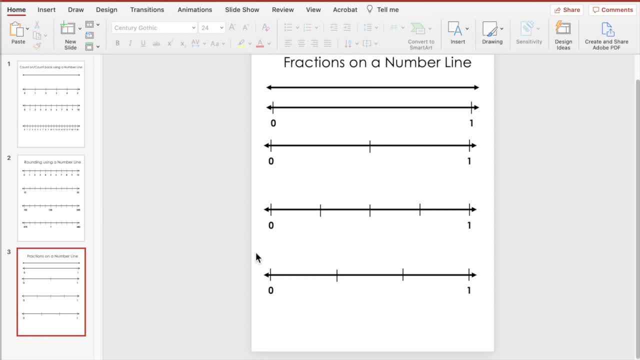 can also extend what they're working on by adding an arrow or a dot. so we're going to add a circle, just like that. hold down the shift button. it'll make that circle equal all around. So then if I put the dot here, let's make it black, with no line. 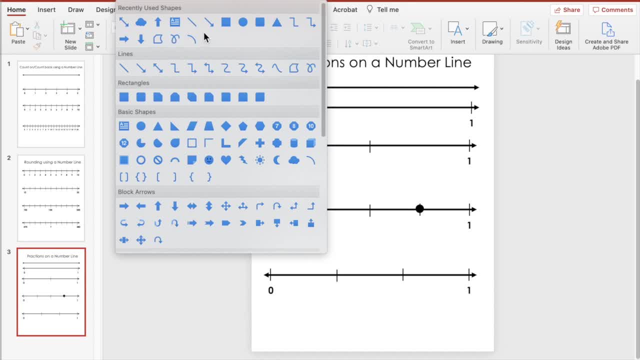 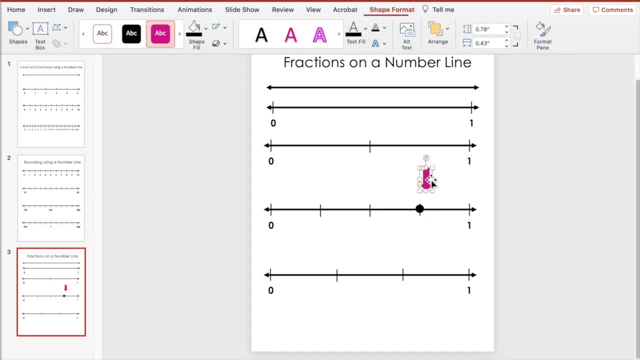 And then maybe put an arrow. go back to my shapes. let's get this arrow here, put that there and then change the color. So then the students would have to identify the point on the number line. So what is that point? what fraction represents that point? 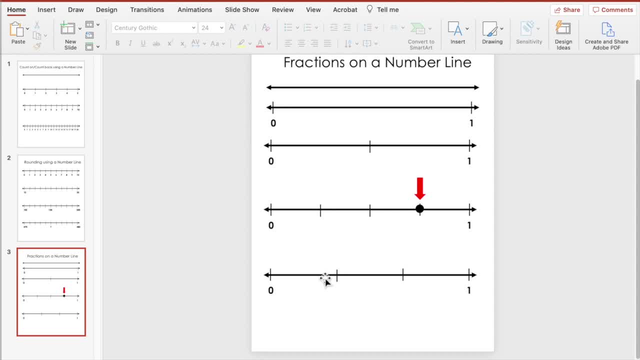 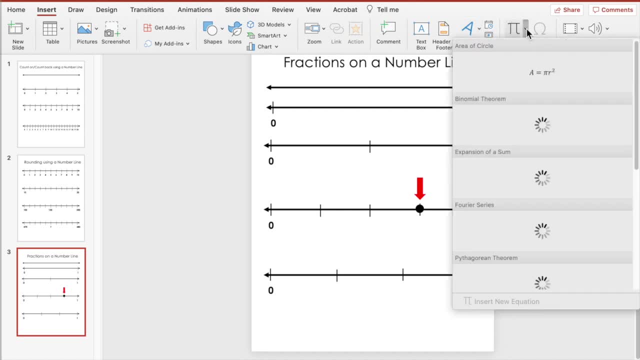 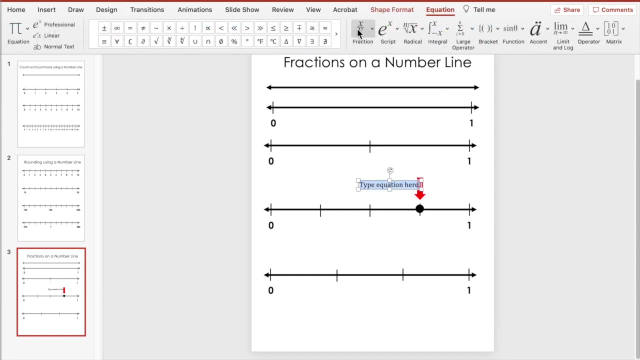 Something else they can do or you can do is insert. when you're doing a text box, you can do: go to insert and add in those fractions. So go to insert equation and then or hit the equation button and then hit the fraction. 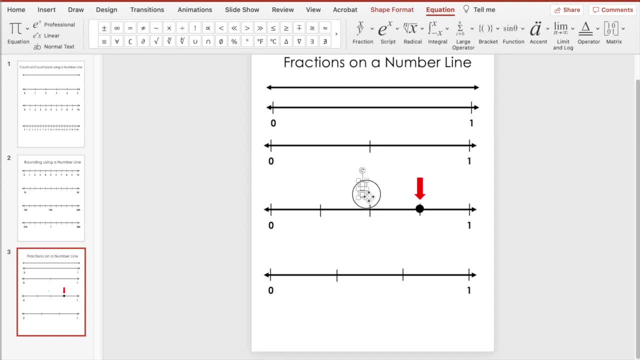 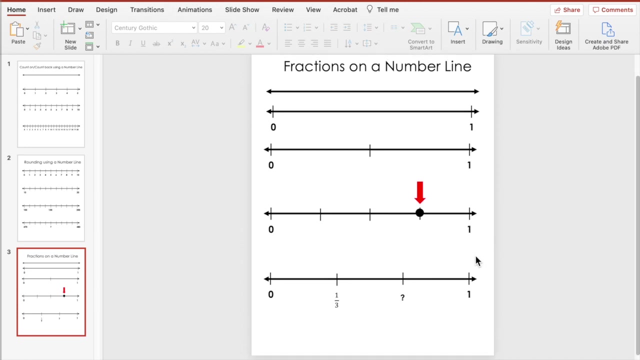 button, hit the one you want and bring that down here and you can put one third and then over here you can just draw like a question mark. so students have to figure out what is the missing fraction. So there are some more examples of what you can do with fractions on a number line. 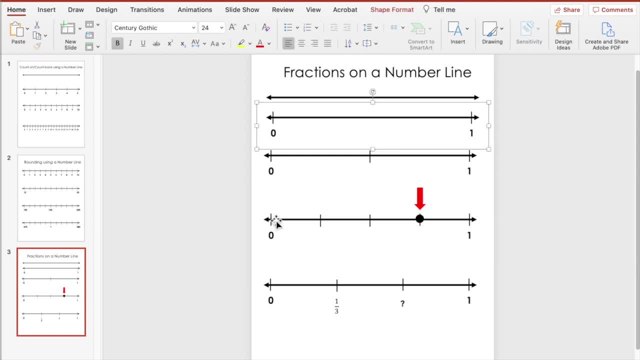 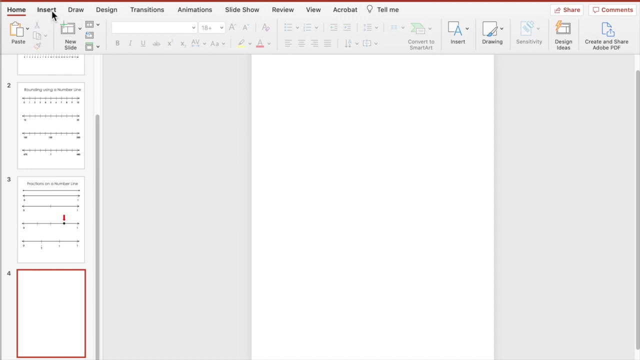 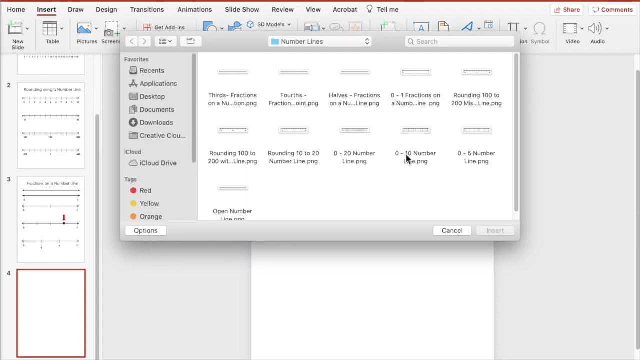 So let's group these and this one will show similar save as picture save, so we have all of those saved as a picture. of course you can print these out, so let's look at how we can insert those pictures. So if I go to insert and then picture, and then picture from file, so I have all of these. 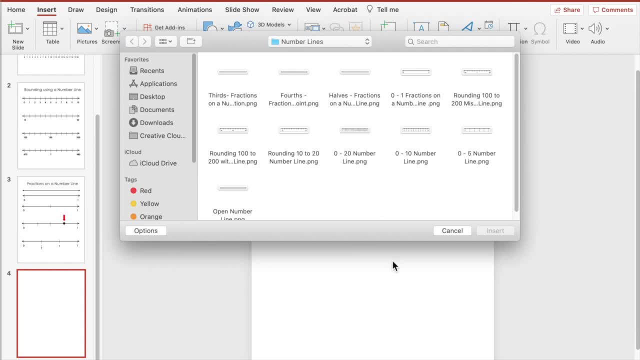 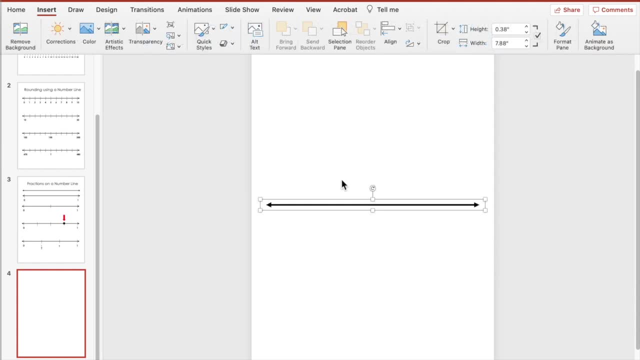 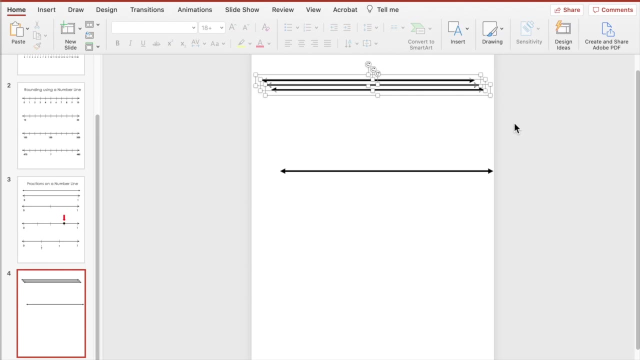 images that I've created and then, because I created them here, they have a transparent background. So if I wanted to give my, if I wanted to create a worksheet with many open number lines, I could do that, or I can just use one. 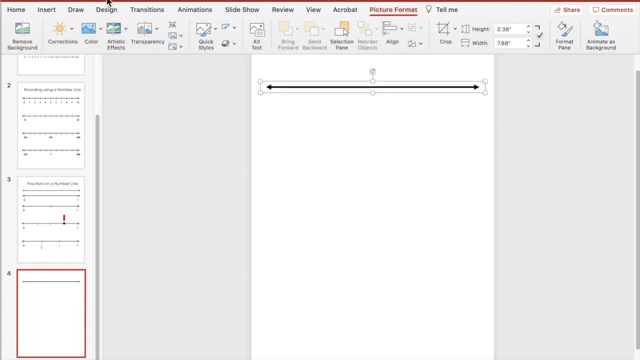 So I'm going to do a number line. let's grab these zero to ten number line. let's grab our rounding one hundred to two hundred So you can put. add that to any page that you want. you can make little flashcards with. 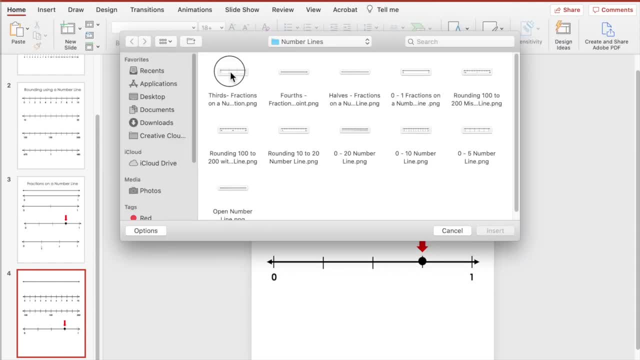 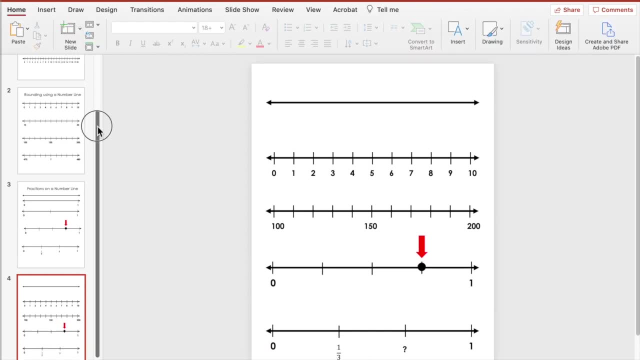 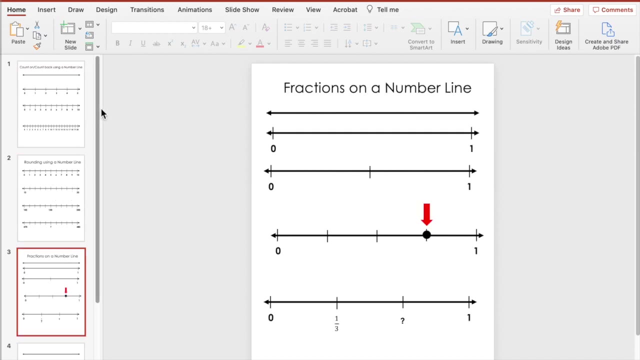 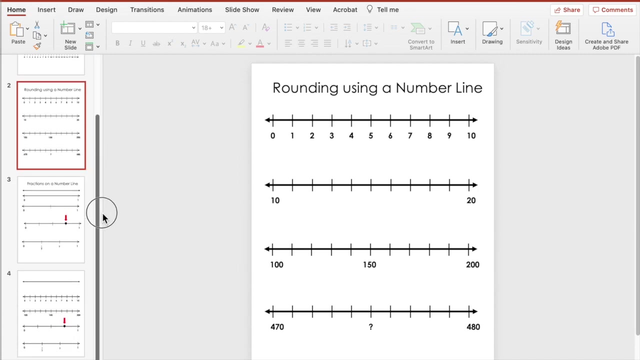 it homework pieces with it. Here we have three different ways that we can use number lines with different math concepts, and I hope this tutorial helped you with showing you how to create your very own number lines to create math resources for your students to work on or your children at home to practice. 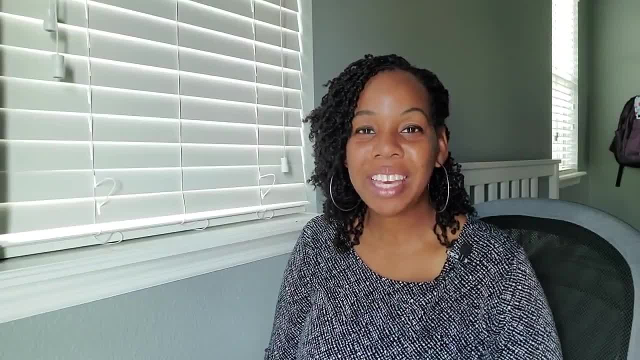 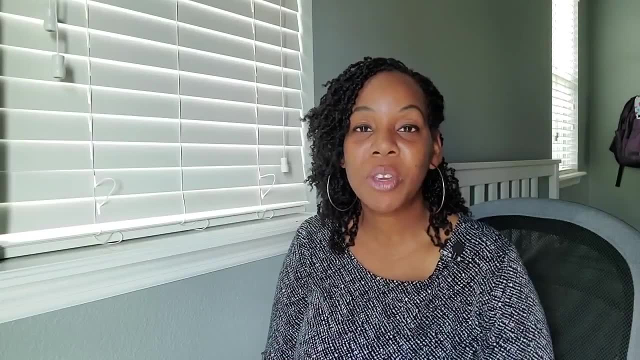 with Okay, day eight is complete. Now you know how to create your very own number lines. There's so many that you can create. You can have students use them as a tool, or you can add them to different pages to create problems for your.